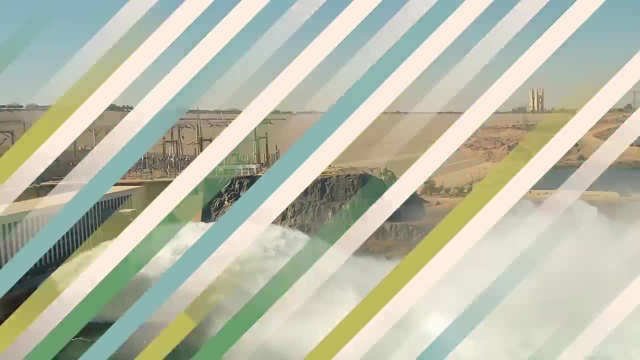 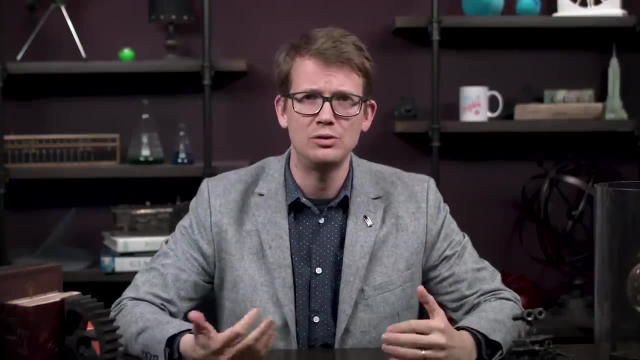 These included many irrigation canals and gigantic dams, like the Aswan High Dam in Egypt, built between 1960 and 1970. These projects allowed people in dry regions or ones subject to seasonal flooding to have more control over when they planted and to grow more harvests per year In the United States. the Reclamation Service, later the Bureau of Reclamation, worked, starting in 1902, to irrigate the western plains. Today that bureau is the largest wholesaler of water in the US. 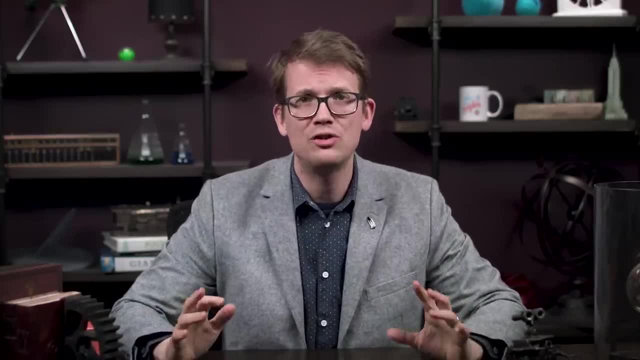 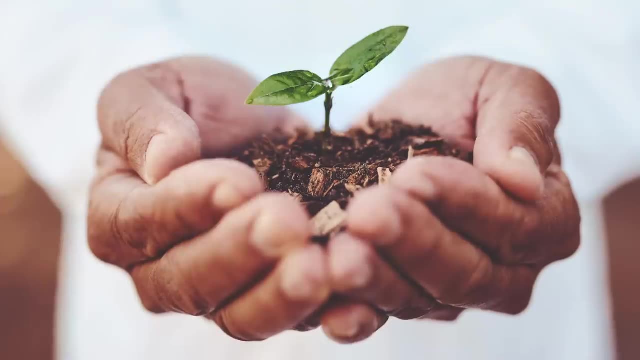 Overall across industrial societies. agriculture changed a lot as engineers developed machines like tractors, chemists created new fertilizers and pesticides, and plant geneticists bred hybrid seeds. Plants need the nutrient nitrogen to grow, but plants can't fix their own nitrogen. from the air, so they need bacteria or human-made fertilizers like ammonia to do it for them, And in the early 1900s German chemists Fritz Haber and Karl Bosch developed a way to take nitrogen right out of the air. 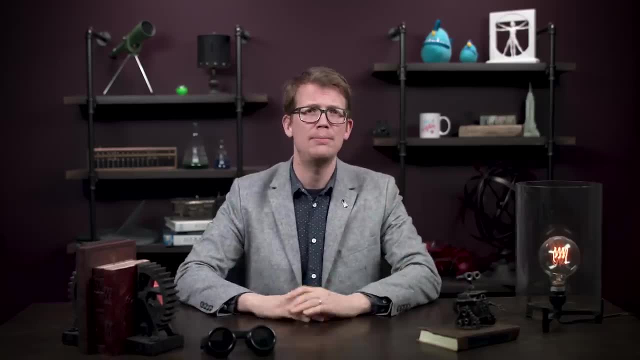 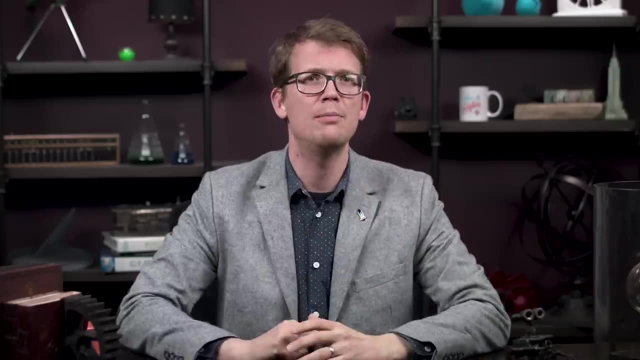 This seemed like a big win. Any industrial society could use the Haber-Bosch process for synthetic nitrogen fixation to make millions of tons of fertilizer and grow more crops. And synthetic ammonia from this process was also used to make nitric acid, which was necessary. 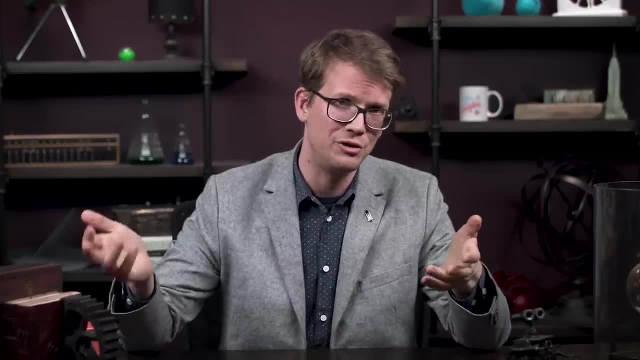 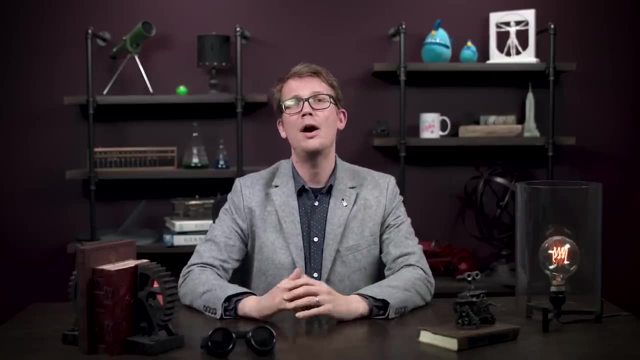 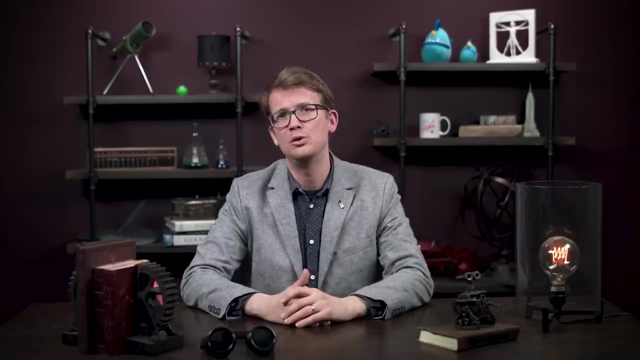 to make explosives. So again, war and professional science were tightly linked. But the bigger problems long-term, were environmental. The Haber-Bosch process requires fossil fuels like oil or natural gas to work, which seemed fine. Industrialists didn't know that burning these fuels would disrupt Earth's climate. 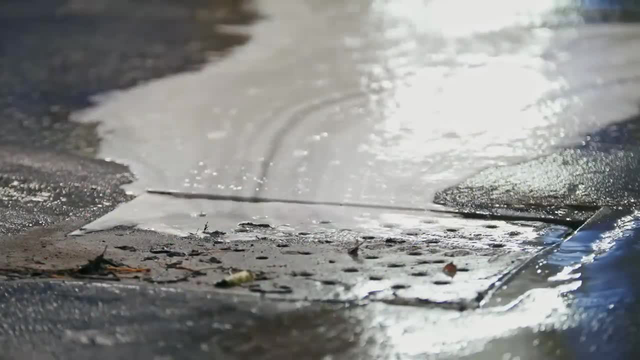 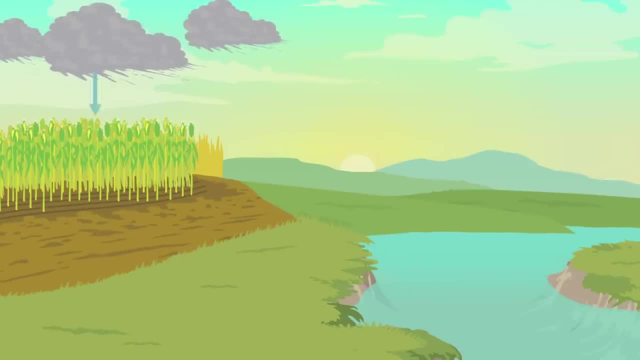 cycles. A more obvious problem is: runoff To make plants take up lots of nitrogen, industrial farming treats them with more fertilizer than they need. Rain washes the leftover fertilizer into waterways, leading to eutrophication, or too many nutrients in the water. 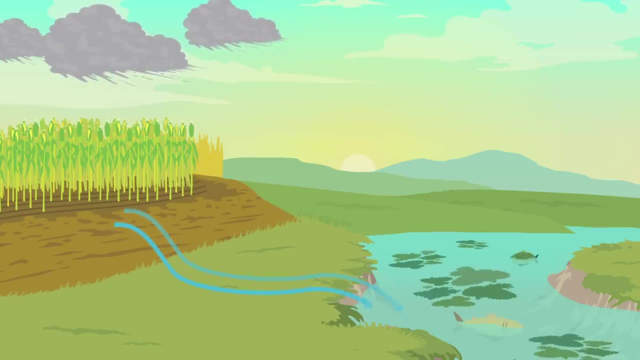 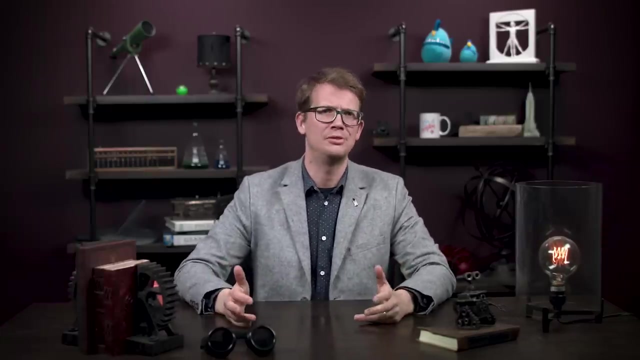 This leads to a buildup of algae which use up all of the oxygen in the water, making it deadly for fish. Another seemingly big win with unintended consequences was an improvement in staple crops. In the 1930s, after decades of research, agricultural scientists in the US rolled out hybrid crop. varieties. These pure strains produced much higher yields, But farmers started using only these seeds. Commercial fields became monoculture or one plant. This means fewer plants are commercially available today and pests can more easily wipe out any one plant. This is the opposite of growing many plants together or polyculture, which can help restore. 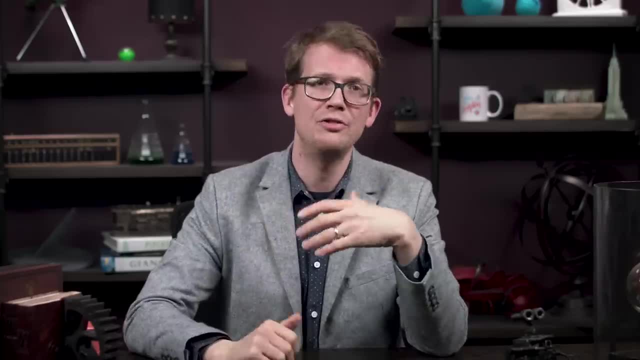 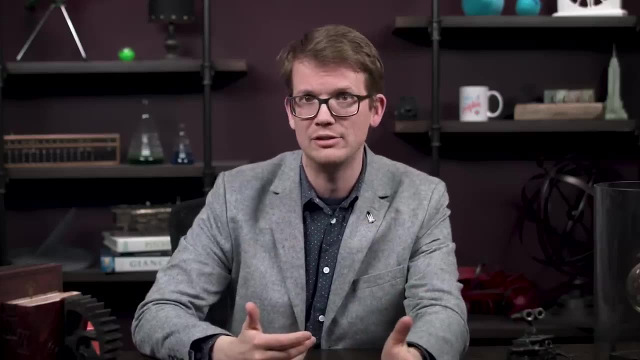 nutrients to soil without synthetic chemicals. So, on the one hand, synthetic fertilizers and hybrid crops seemed like easy wins. On the other hand, there were negative consequences. So what's next? There were negative long-term consequences. And also, on the third hand, even these advancements didn't prevent environmental problems and 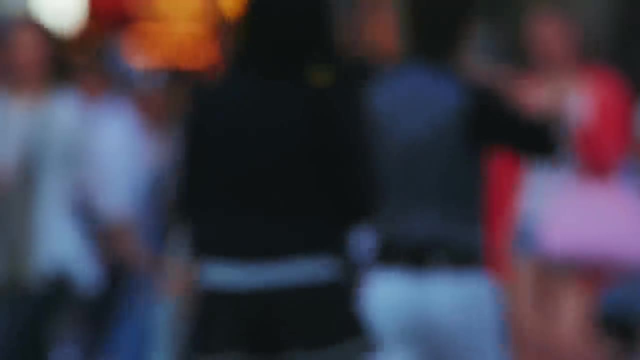 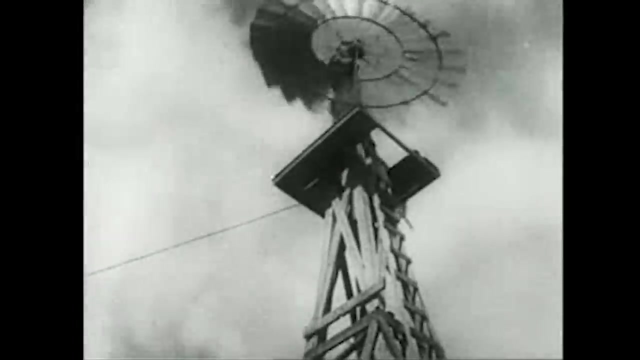 growing fears that agricultural innovation just couldn't keep up with rapid population growth. For example, part of the US experienced severe droughts in the 1930s and was farmed in unsustainable ways. This led to massive dust storms, collectively called the Dust Bowl, which forced many farmers 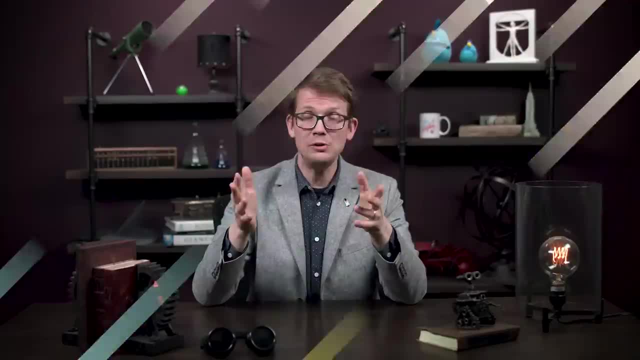 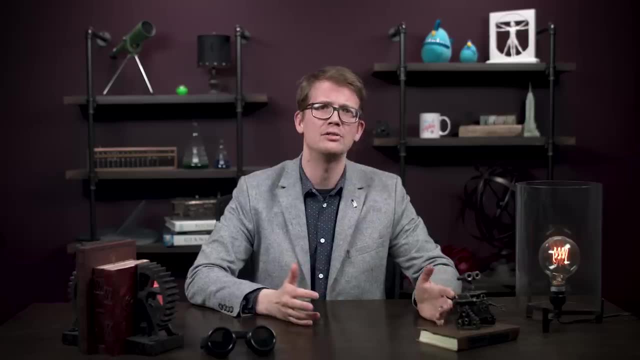 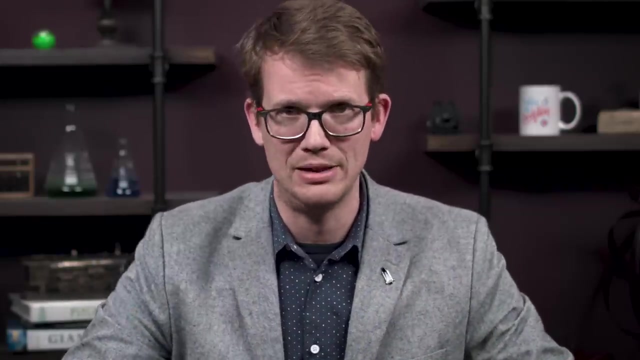 to abandon their farms. during the Great Depression, And this was the United States. At the time, most of the world's farmers remained smallholders. They worked plots of land smaller than 10 hectares, largely without industrial machines. Populations were growing, but storms and wars threatened to lead to famines. 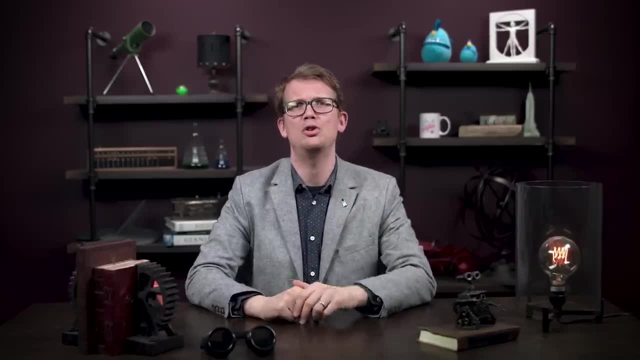 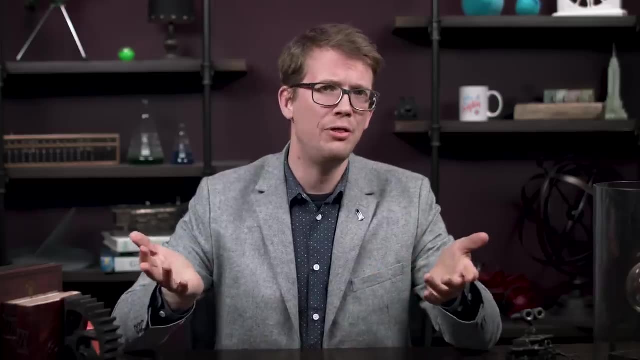 So many scientists taking a note from that crotchety preacher who inspired Darwin, Thomas Malthus wrote pessimistically about humanity's future. Probably the most famous of these Neo-Malthusian thinkers was American biologist Paul Ehrlich, whose 1968 bestseller The Population was published in the New York Times. 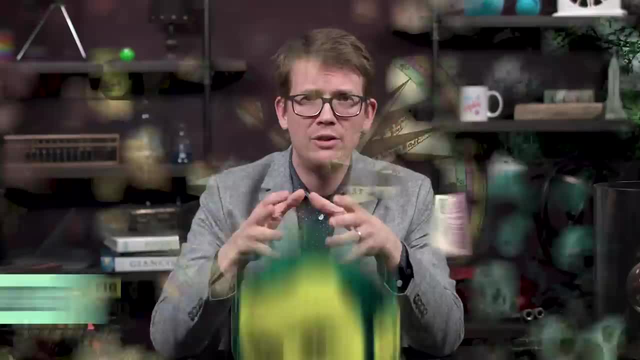 He wrote: The Population was published in the New York Times. He wrote: The Population was published in the New York Times. A Cloud Population Bomb predicted that famines would soon kill millions of people, especially in India, Which didn't happen. 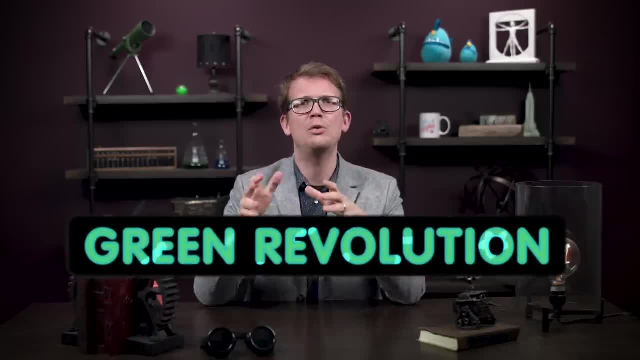 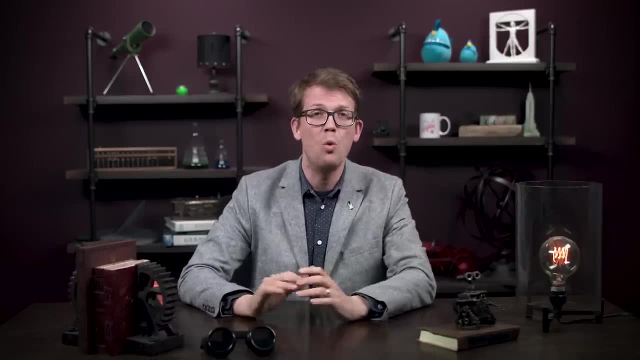 Arguably the biggest example of humans controlling our environment was the Green Revolution in the 1950s and 60s, when crop yields went up for farmers in less industrialized countries Way up. In one sense, it's a simple story of science applied. 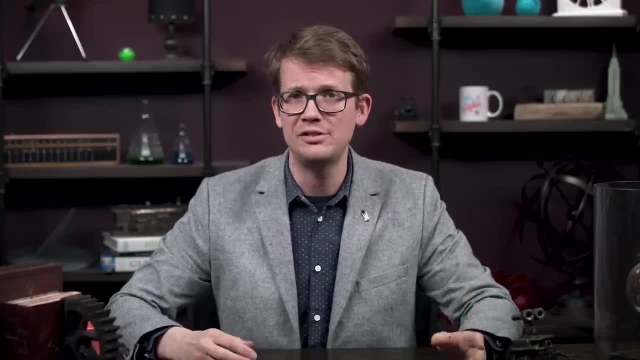 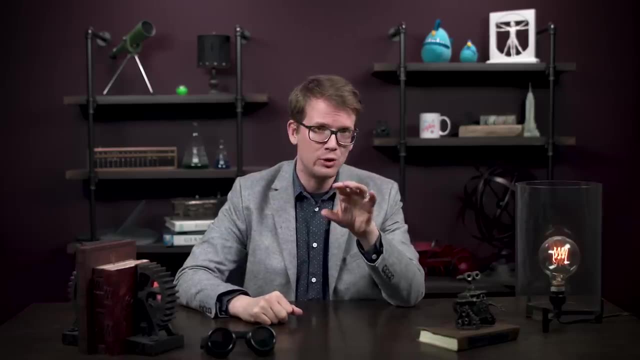 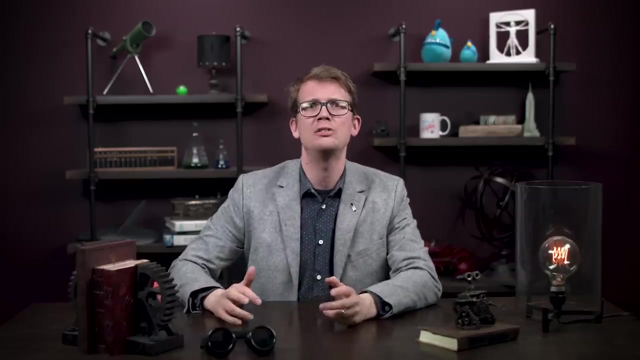 Scientists from rich countries offered new techniques built on hybrid seeds. In another sense, it's science in the service of policy. This revolution was organized by International Agricultural Research Centers, or IARCs, which were funded by federal grants from developed and developing countries and by private foundations. 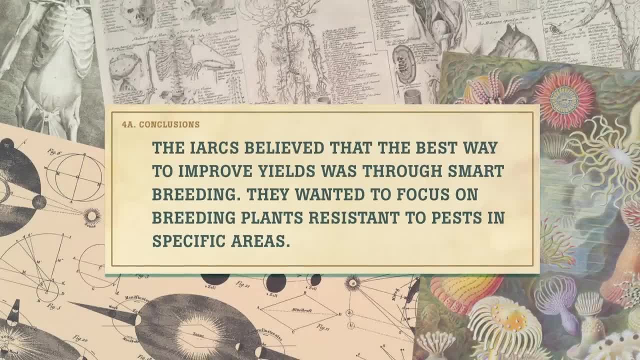 like Rockefeller and Ford, The IARCs believed that the best way to improve yields was through smart breeding. They wanted to focus on breeding plants resistant to pests in specific areas and simultaneously to make these plants take up more nitrogen and grow more edible material. 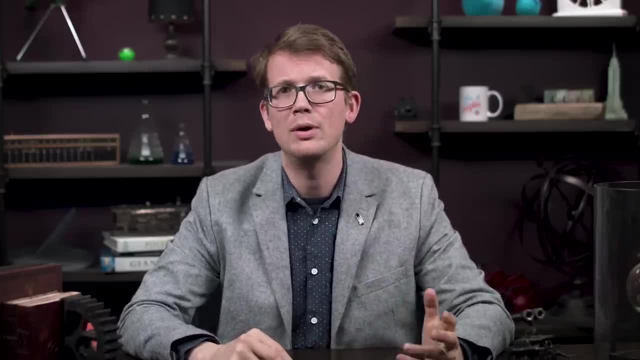 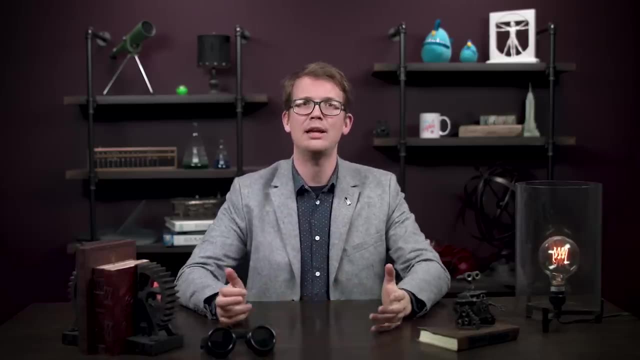 Lots of people were involved in this work, particularly in the US, Mexico and India. But people love heroes, so Green Revolution stories often focus on American agronomist and plant geneticist Norman Borlaug, who was, to be fair, an awesome scientist. 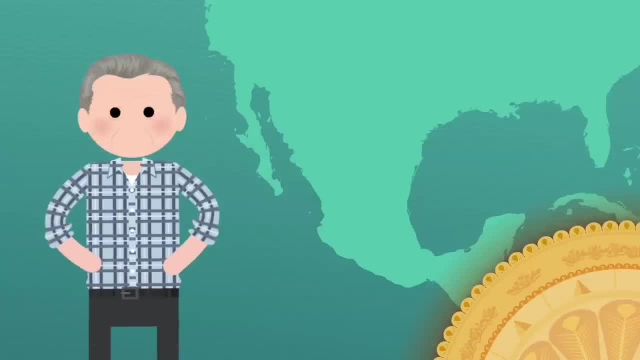 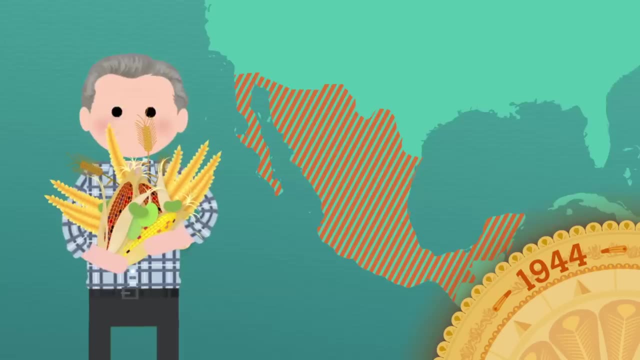 Thought Bubble introduce us. Borlaug joined the Rockefeller Foundation's group in Mexico in 1944. He had never worked on wheat, maize or beans before And he didn't speak Spanish, But he eventually learned it and stayed in Mexico. 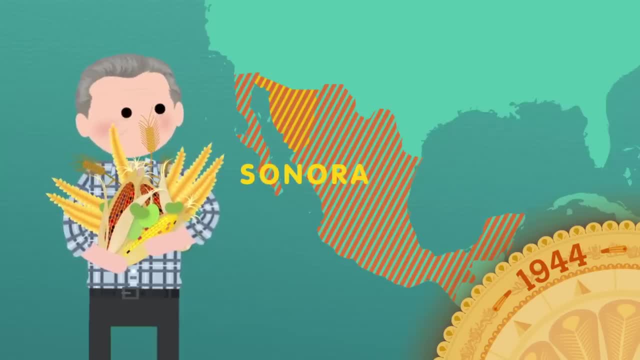 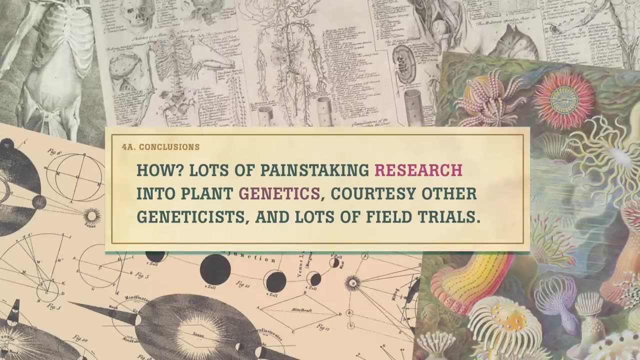 He lived in Mexico for 16 years, working mostly in Sonora. He developed a hybrid wheat that withstands a common fungus called rust blight. How Well: lots of painstaking research into plant genetics, courtesy of other geneticists, and lots of field trials. 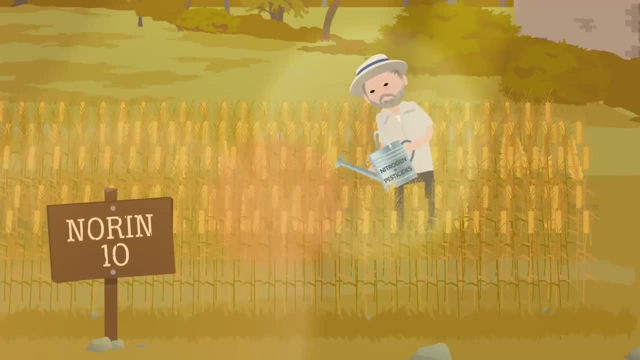 Borlaug took Norin 10,, a wheat bred by Japanese scientist Gonjiro Inazuka that was short but produced lots of food if given lots of nitrogen and defended with chemical pesticides, and bred a semi-dwarf wheat specifically for Mexican climates. 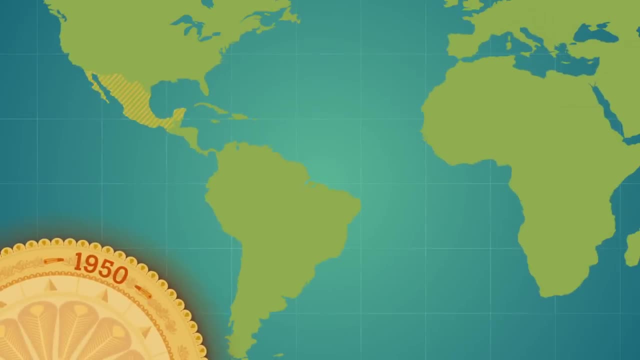 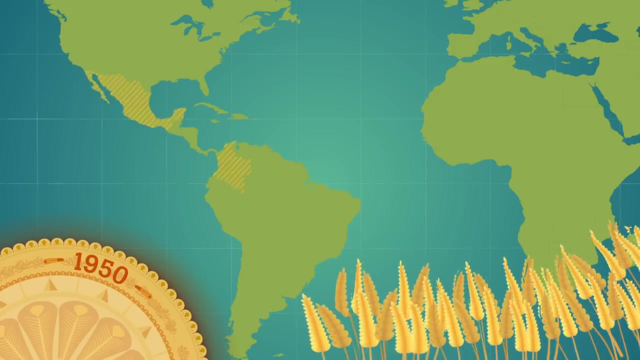 Starting in the 19th century, Borlaug was the first scientist to produce wheat. Then, around 1950,, Mexican agriculture shifted toward high-yielding varieties of wheat, synthetic nitrogen and pesticides, And this revolution in farming soon spread to Colombia, Chile and India. 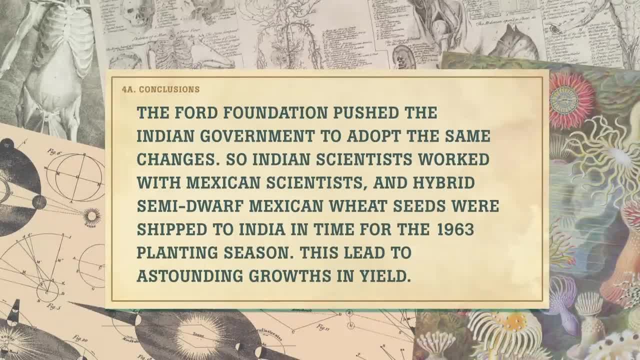 The Ford Foundation pushed the Indian government to adopt the same changes. So Indian scientists worked with Mexican scientists and hybrid semi-dwarf Mexican wheat seeds were shipped to India in time for the 1963 planting season. This led to astounding growths in yield. 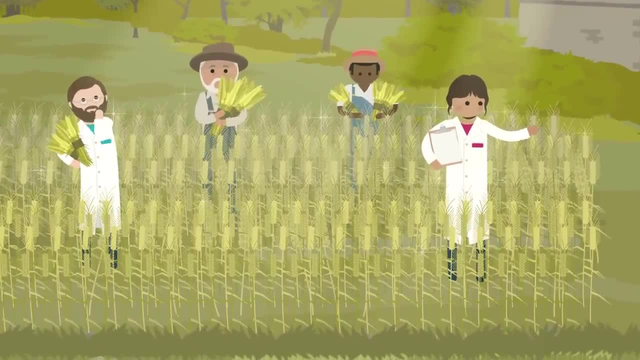 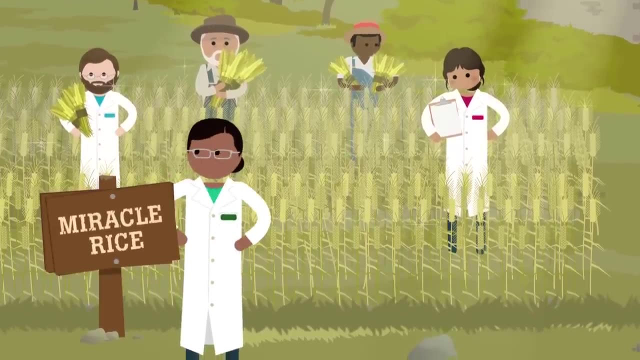 Also in the 1960s, an international team of scientists and scientists from the United States worked to develop a new variety of high-yielding semi-dwarf rice called IR-8, sometimes called Miracle Rice. In 1971, the Rockefeller and Ford Foundations created the Consultative Group on International 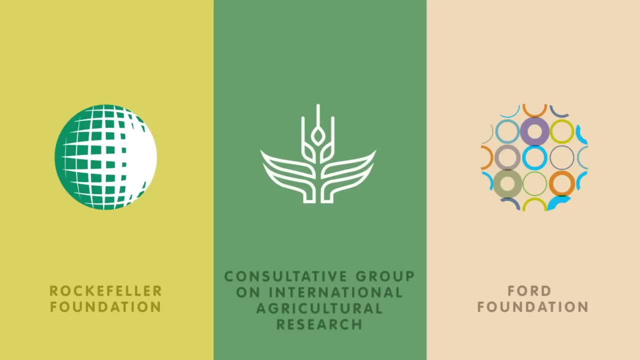 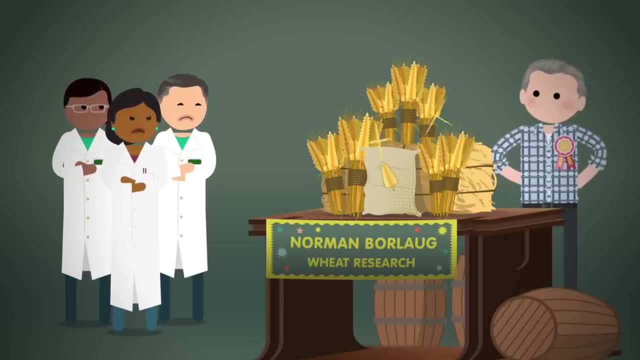 Agricultural Research to further extend the IARC research. Borlaug won the Nobel in 1970, but no Mexican, Indian or Japanese scientists shared the prize. Thanks Thought Bubble. Meanwhile, with minimal support from the Soviet Union, the map of the world has become more. 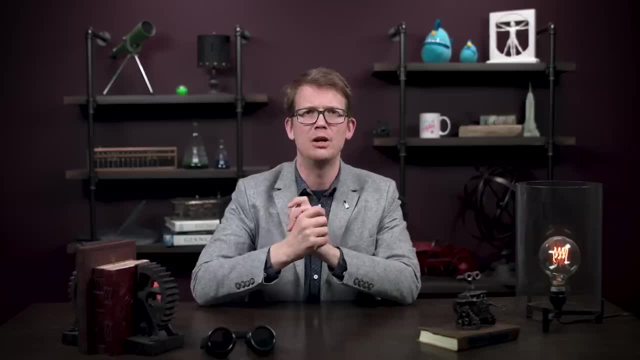 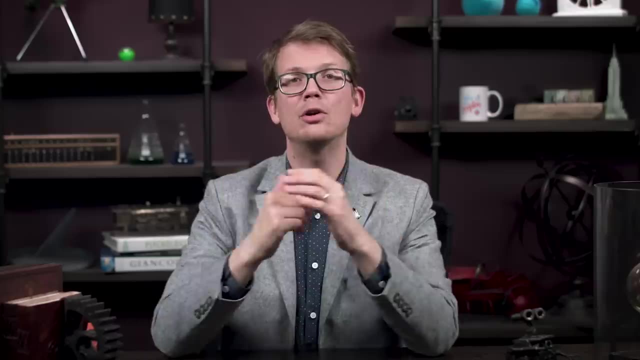 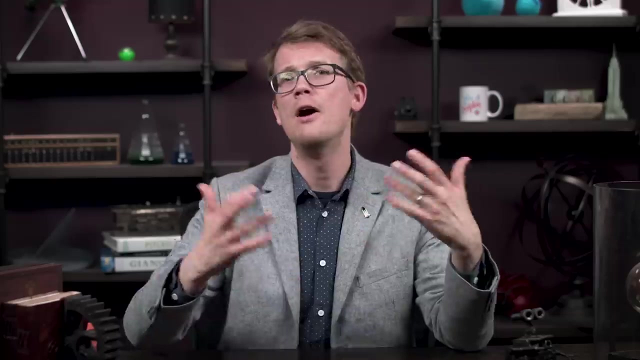 clear. The Green Revolution in the Maoist Chinese state fostered its own scientific farming, including a system of experimental agricultural stations and hybrid sorghum and hybrid rice varieties. Agriculturally, the Green Revolution was an immediate success. Thousands of tons of seeds moved from Mexico to India. food prices dropped. India became 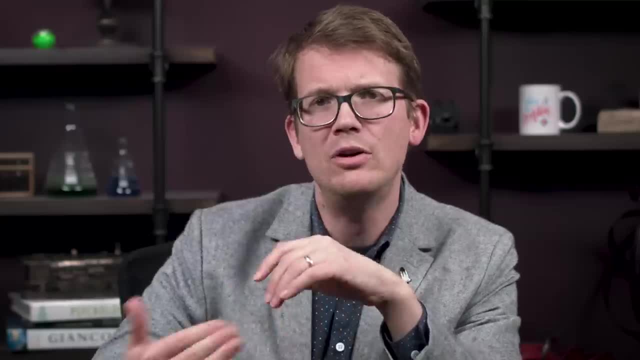 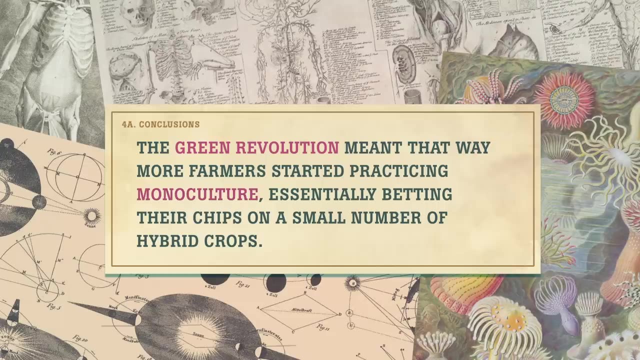 a rice exporter and currently overproduces wheat. But in the longer term, the Green Revolution meant that way more farmers started practicing monoculture. They started essentially betting their chips on a small number of hybrid crops. Thousands of traditional varieties are no longer cultivated. 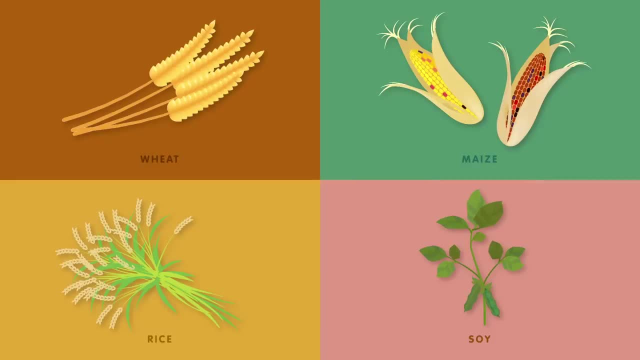 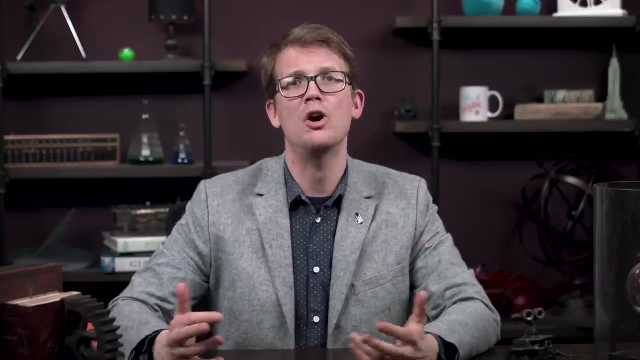 Only four crops — wheat, maize, rice and soy — provide more than half of our food today. Socially, industrial farming requires investing in expensive equipment and hybrid seeds which aren't produced by the previous year's harvest. This changed the business cycles of farmers. Zooming out. the Green Revolution changed what defines a modern society. It now meant using synthetic nitrogen. It changed the environment. It changed agriculture. It changed agriculture. It changed food production: pesticides and tractors on large monoculture farms. The idea of the Revolution had been to end hunger and it probably prevented millions. 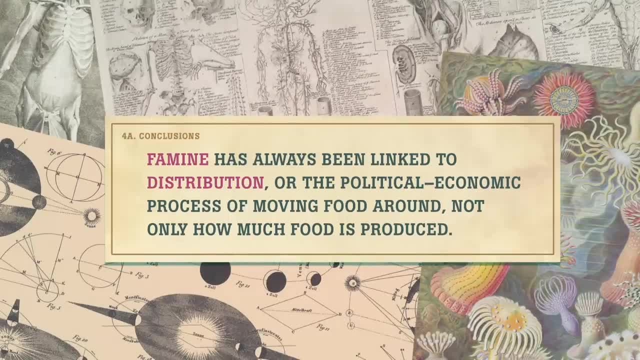 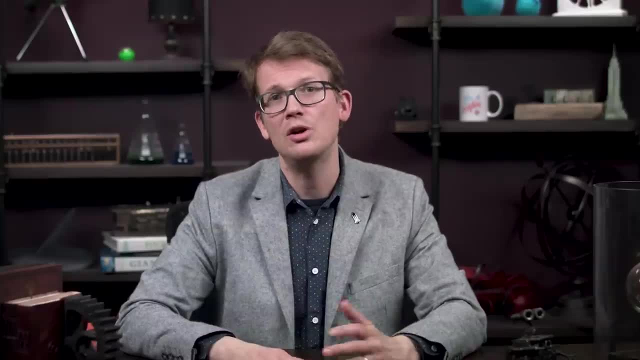 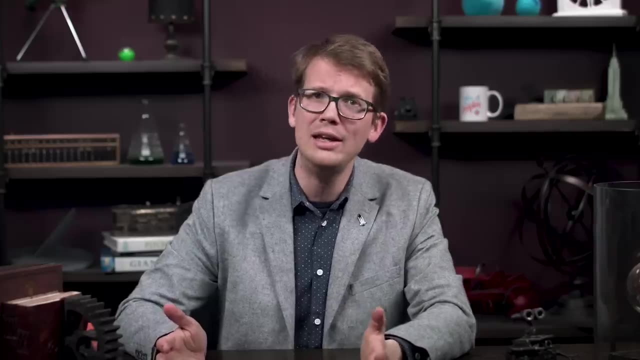 from starving. But famine has always been linked to distribution or the political-economic processes of moving food around, not just to how much food is produced. And the Green Revolution was also always about the United States flexing its scientific muscle around the world, buying allies with bread, including India, the world's largest democracy. 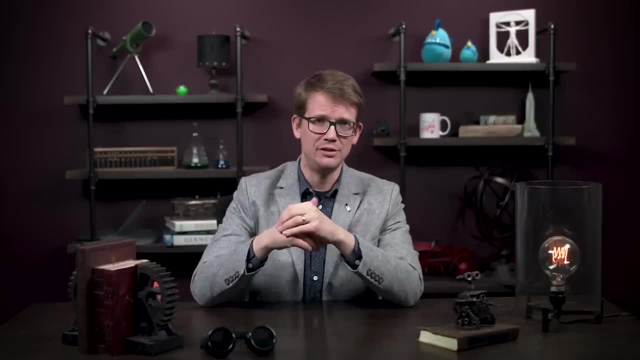 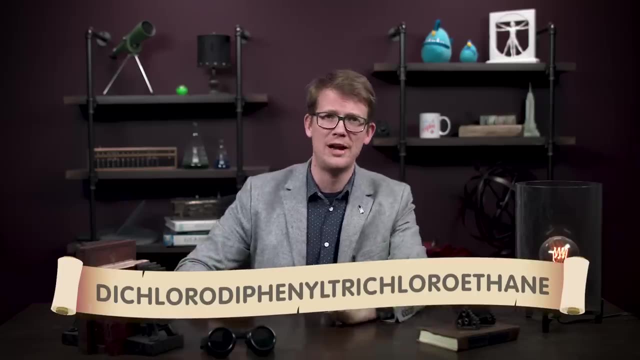 This is soft power. Meanwhile, also in the 1950s and 60s, synthetic pesticides were used to control bugs that spread human illnesses. The most famous was dichlorodiphenyltrichloroethane, which you probably have heard of as DDT. so 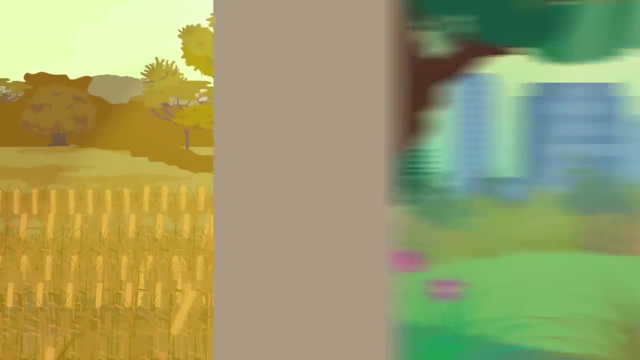 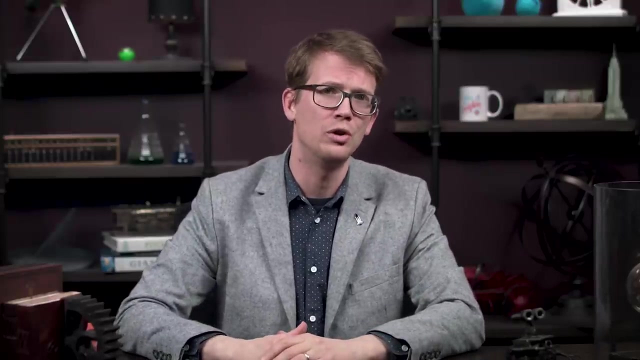 that you don't have to say that whole thing. That was spread on fields and urban green spaces, right on the little kids just everywhere. It had seemingly miraculously dropped mosquito populations during World War II, helping fight the spread of malaria and typhus. 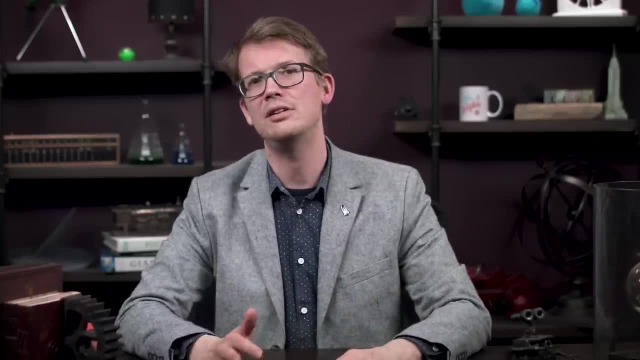 Only it turned out that DDT, while not as effective as the DDT, was not as effective as the DDT. It was not as effective as the DDT And, while not immediately toxic to humans, it was toxic to lots of other living things. 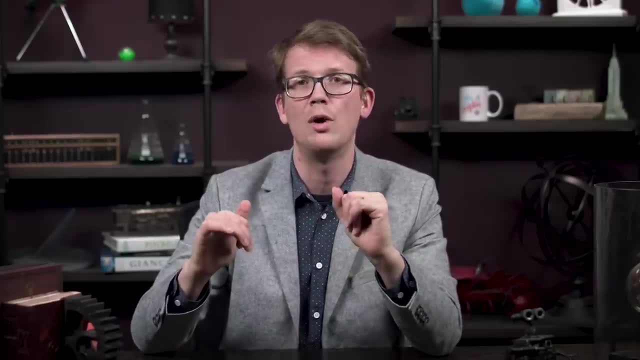 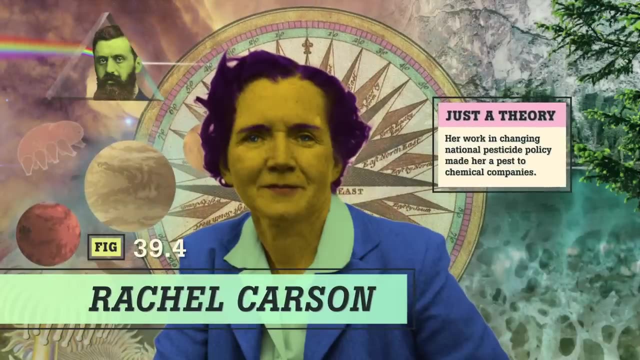 like birds and fish, And it wasn't good for humans in the long run either. After years of careful research, all of which angered scientists working for the chemical industry, American biologist and pioneering environmentalist Rachel Carson wrote a series of articles that became the book Silent Spring in 1962. 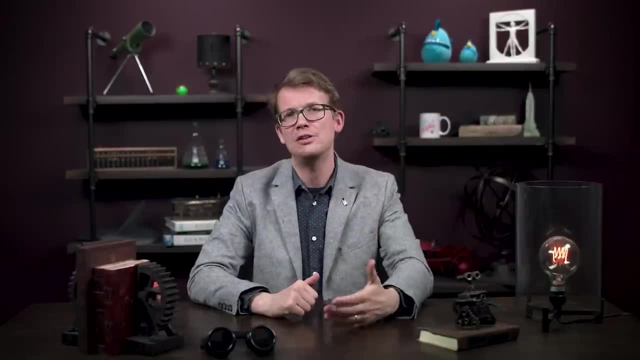 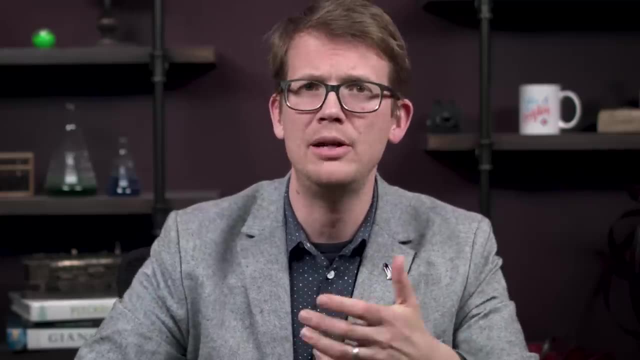 She explained in simple, beautiful language how some kinds of synthetic pesticides work and why they are often a terrible idea. In this book, along with her other books, numerous op-eds and appearances, Carson helped spark the modern environmentalism movement in the United States. 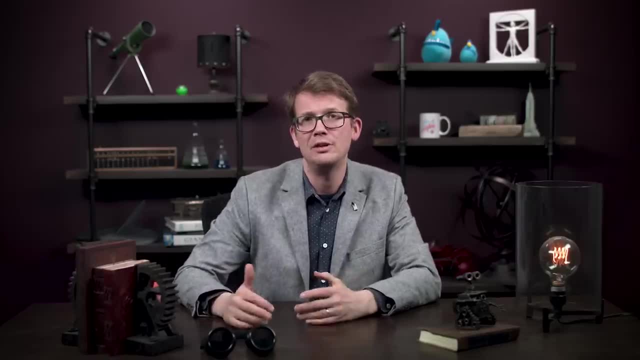 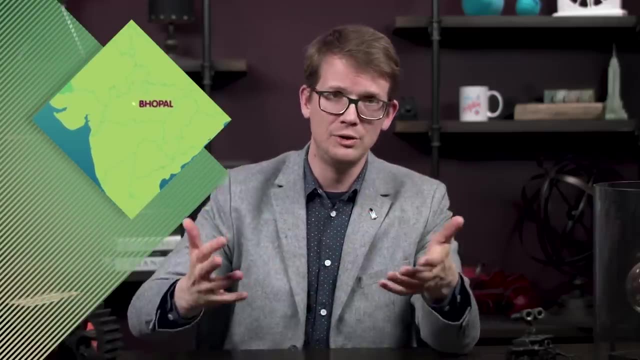 In addition to long-term effects, pesticides have also been involved in acute disasters. In 1984, a Union Carbide India chemical plant in the city of Bhopal had a serious accident. This plant produced the insecticide 7, using a highly toxic chemical called methyl isocyanate gas. The accident released 32 tons of methyl isocyanate. Half a million people were exposed. 4,000 people died immediately. 2,500 died that year. Bhopal is widely considered as the worst industrial disaster in history. Only two years later, in 1986, the Chernobyl reactor melted down in Ukraine. Clouds of radioactive material billowed across Europe and then the world, Conflicting politically-inflected epidemiological studies put the long-term casualties from cancer due to Chernobyl at anywhere between 10,000 and hundreds of thousands. So… The disaster hasn't been a total slam-dunk for humankind. 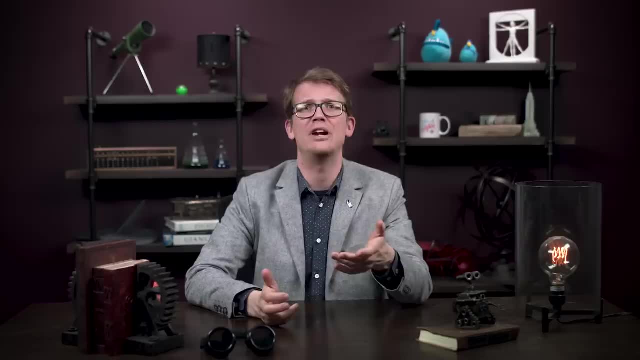 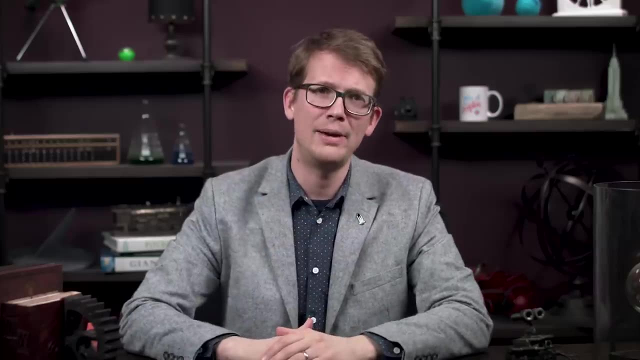 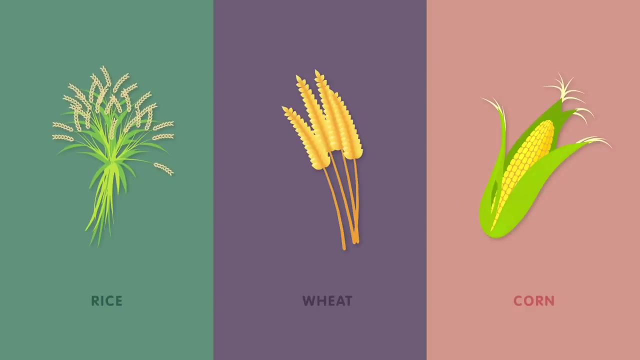 And most of humankind has had no say in these projects. The effects, good or bad, just happened to them, And this is still the case. In fact, the Intergovernmental Panel on Climate Change warns that global food supplies are in danger because staple crops like rice, wheat and corn are now facing a slowdown. 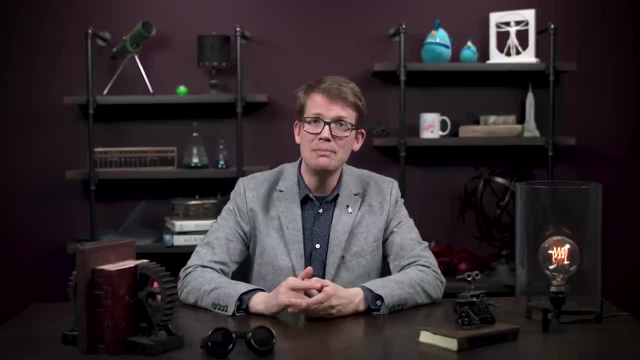 in the rate at which their yields go up, Meaning back to Malthus: we might soon have more hungry mouths than food, even if agronomists keep making them. But that's not all. There's still a long way to go before we can keep making incremental gains. 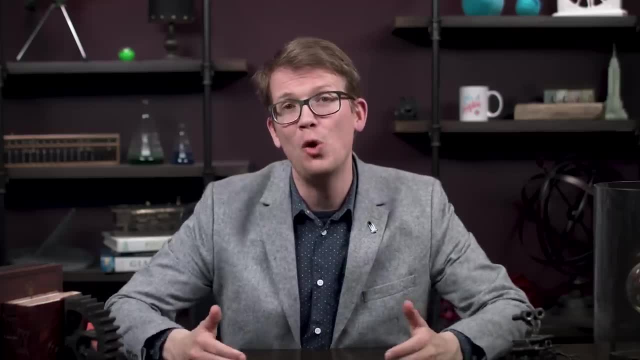 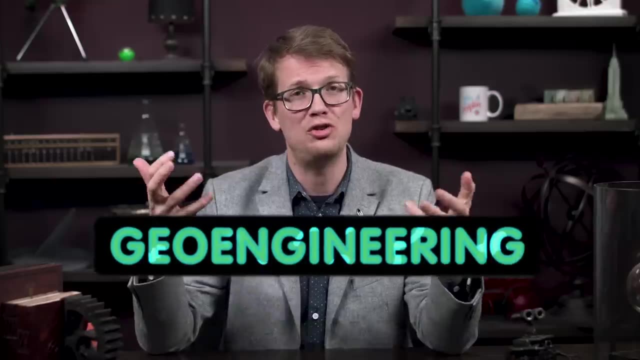 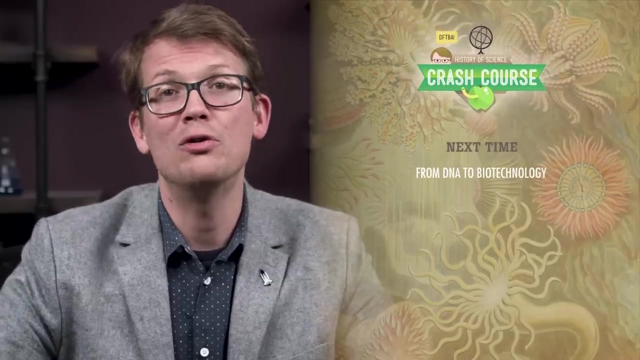 So some serious scientists are returning to the idea of controlling the climate. In 2006,, Nobel-winning atmospheric scientist, Paul Krutzen, called for humanity to use geoengineering- the modification of the climate- to keep our world habitable. Next time we'll look at control over living things at a different scale. 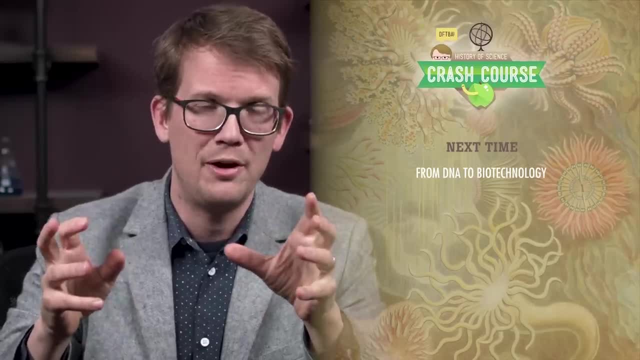 It's the characterization of DNA and the birth of biotechnology. Crash Course History of Science is filmed in the Dr Cheryl C Kinney Studio in New York. It's a great place to be. It's a great place to be. It's in Missoula, Montana. 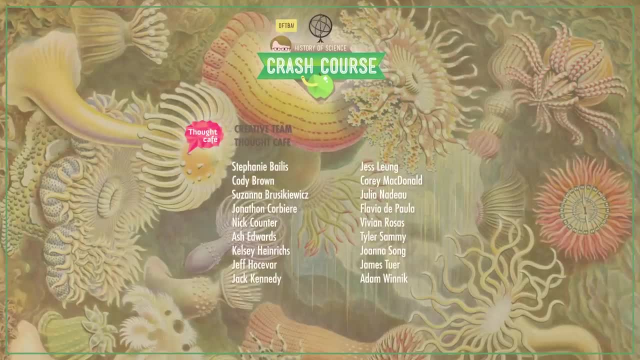 And it's made with the help of all of these nice people, and our animation team is Thought Café. Crash Course is a Complexly production, If you want to keep imagining the world complexly with us. we've got a bunch of other shows. 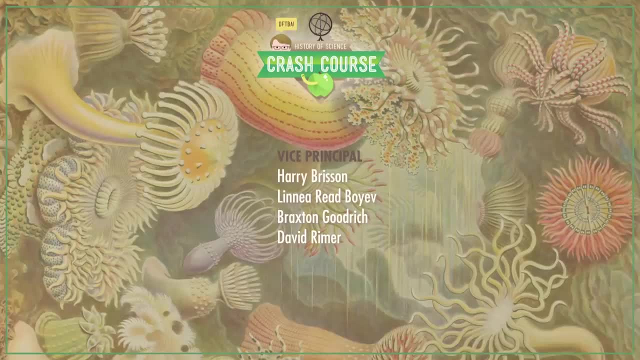 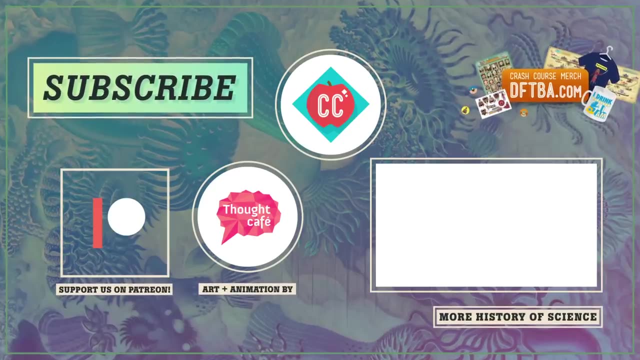 that you can check out, like Nature League, Sexplanations and, of course, SciShow. And finally, if you'd like to keep Crash Course free for everybody forever, you can support the series at Patreon, a crowdfunding platform that allows you to support the content. 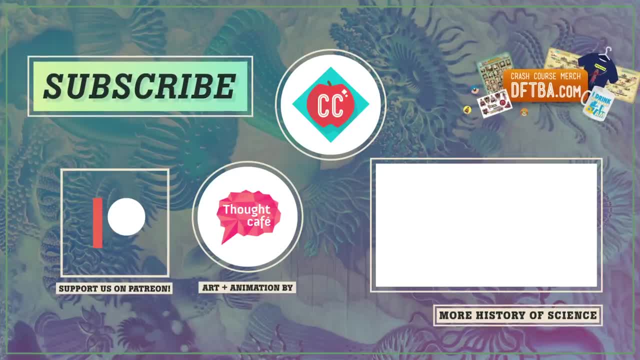 you love. Thank you to all of our patrons for making Crash Course possible with your continued support. We'll see you next time. Bye.